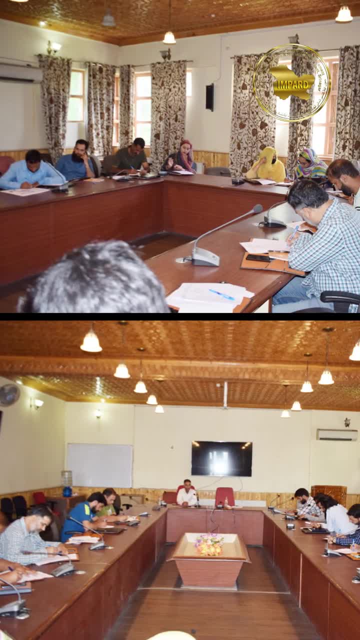 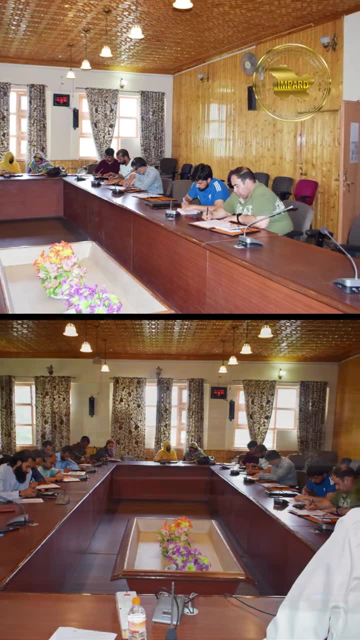 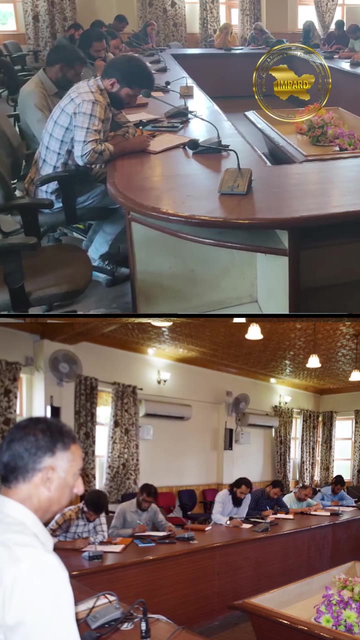 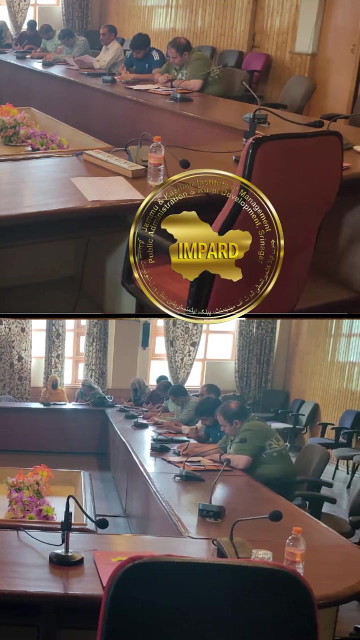 The video is not suitable for all audiences. Please note that the video is not suitable for all audiences. 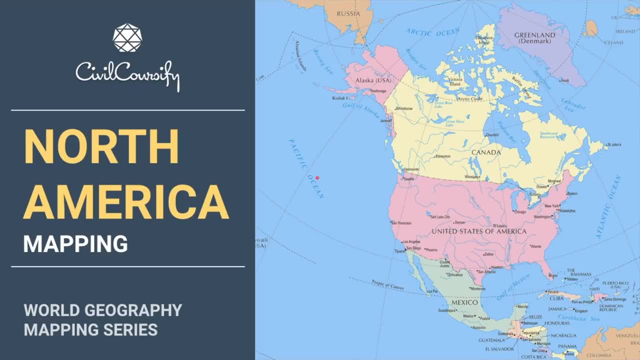 Hello everyone, in this video we are going to map the continent of North America. Now, this video series is very important because you'll get a lot of questions from various maps- either India or the world, So make sure that you have your atlas with you. 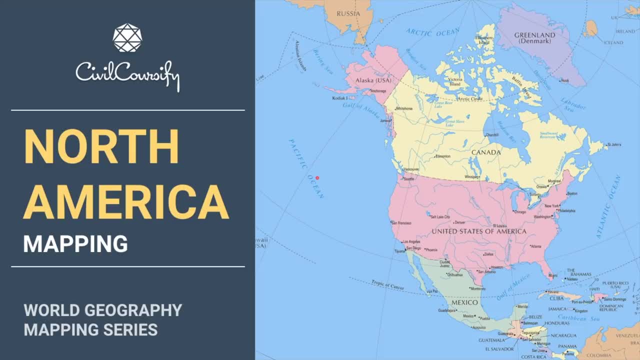 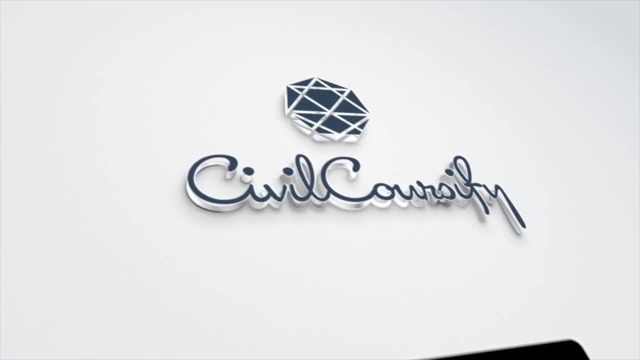 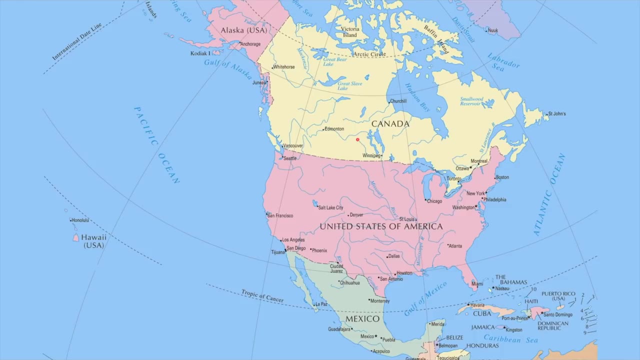 either Orient, Blackspawn or Oxford, so that you can map side by side and eventually finish off the entire part instantly. Alright, let's begin Right. so in this video we will cover the countries of North America, such as Canada. then we have the United States of America and Mexico. We will cover the southern countries. 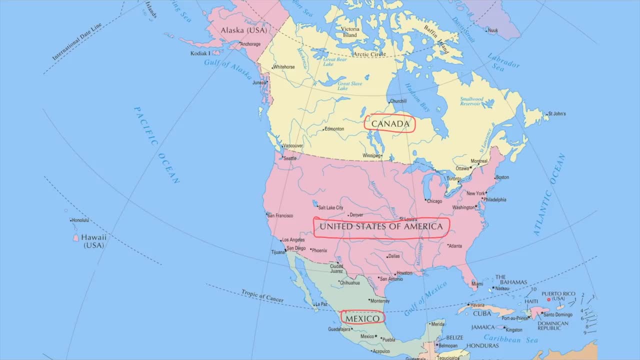 from Mexico in the Central America part, and along with that we will also cover the Caribbean Islands in the same video. Right? so Alaska, as you can see here it is a part of Europe, Right? so in this video we will cover the countries of North America, such as Canada. 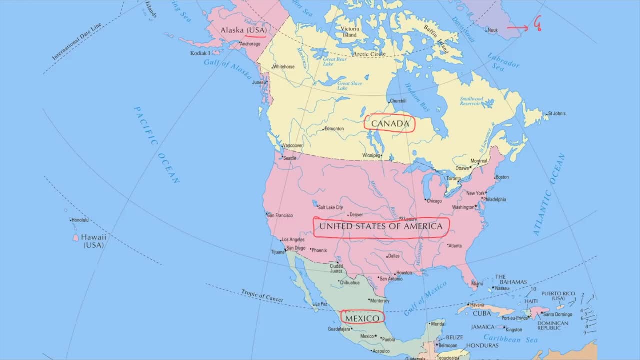 USA only. Along with that, we have Greenland, which is a part of Denmark. Now let us quickly revise some water bodies surrounding this landmass, Although we have covered the water bodies in the previous video, the overview one, but still let's take a look. This is the Pacific Ocean on the western side of this. 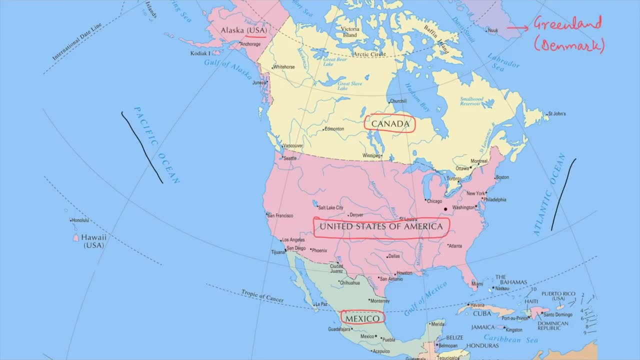 continent and this is the Atlantic Ocean on the eastern side of North America. This is the Gulf of Alaska, and then we have the Gulf of Mexico. This is the Bering Sea between Alaska and Russia. This is the Beaufort Sea in the Arctic Circle. Then we 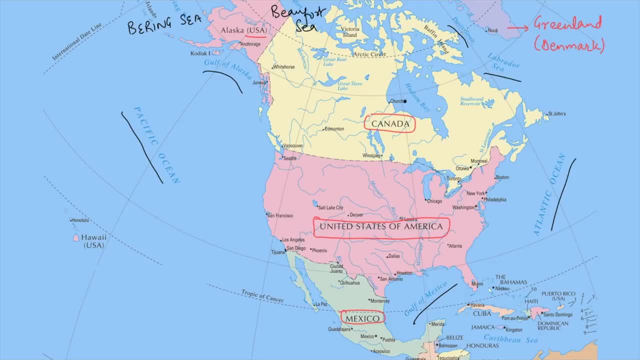 have the Davis Strait in the Arctic Circle. This is the Labrador Sea. In Canada, we have the Hudson Bay. So these are the major water bodies in or around this continent. We will now look at the rivers and lakes. Now, this is the Gulf of California. Now, when we talk,